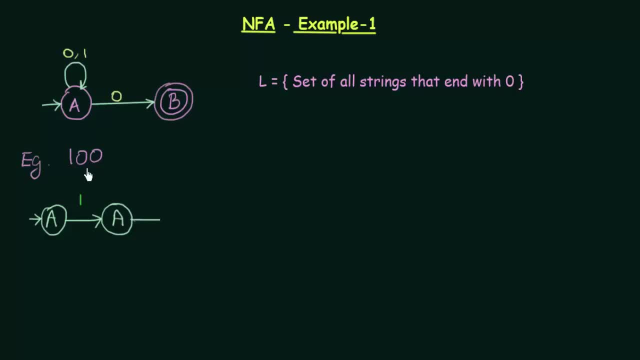 We see from here. And then what is my next input? My next input is 0.. My next input is 0,. this one. So, on getting input 0, where does A go? A goes to A itself and also A goes to B. 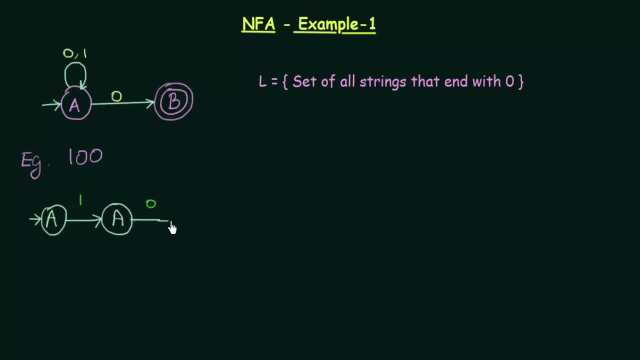 There are two transitions. A. it can go either to A itself Or it can also go to B. There are two transitions. A goes to either A or B on getting input 0.. Alright, Now we are in these two states. 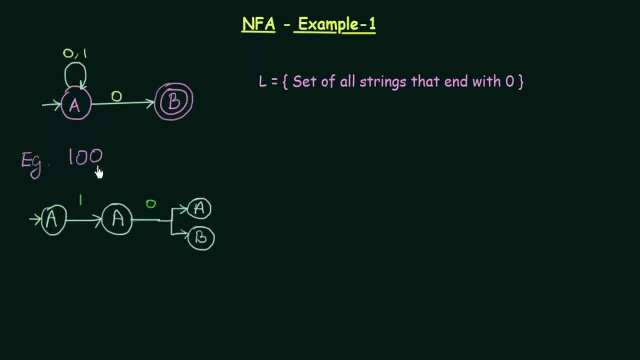 Right, And what is my next input? My next input is again 0.. My next input is again 0.. And what happens? Let us see: A on getting input 0, where does it go? A on getting input 0, it goes to A. 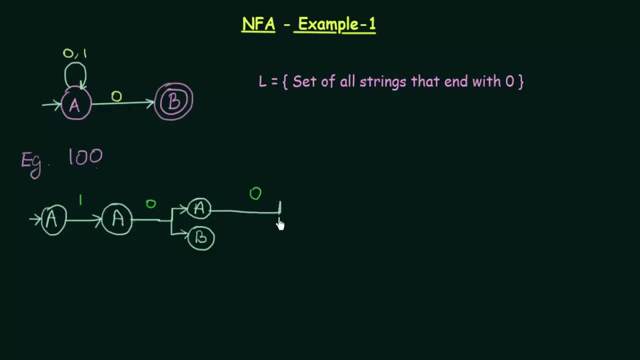 And B right A on getting this input 0.. Again, it goes to A itself Right here And it also goes to B. It also goes to B. And what about B? I am in two states over here, So I have to check for both the states. 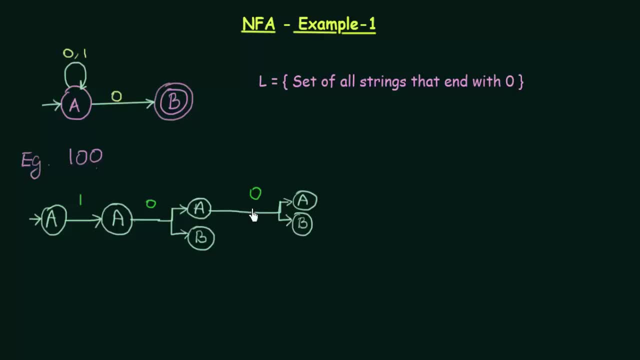 So A on getting this input 0, it went to A and B. And what about B? B on getting input 0, where does it go? B on getting input 0, it goes nowhere. There is nothing mentioned. Means A goes nowhere. 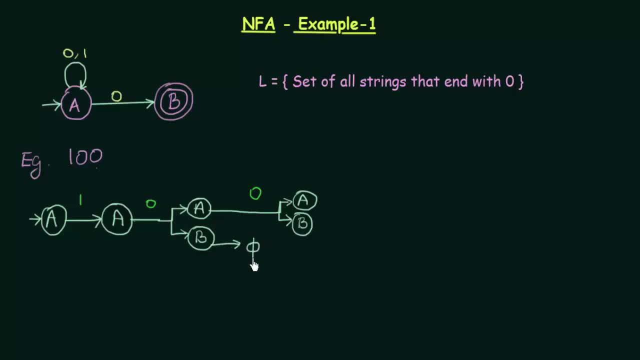 So I will say that it goes to 5.. Right A does not go anywhere. Now, is this accepted or not? How do we know At the end of the string, that is, at this 0, 1, 0, 0,, when I reach the end of the string? 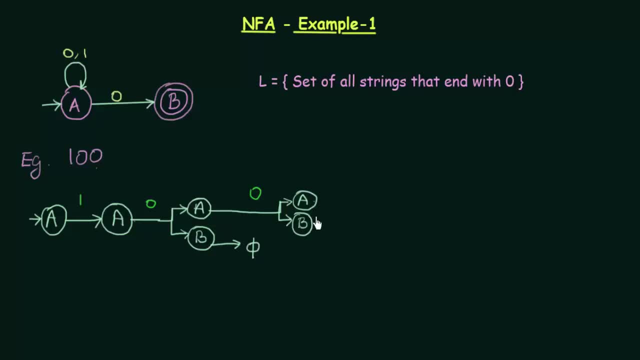 what is my current state? I am in A- B. Is A an accepting state or final state? No, A is not, But is B an accepting state or final state? Yes, B is an accepting state or a final state, So this string will be accepted. 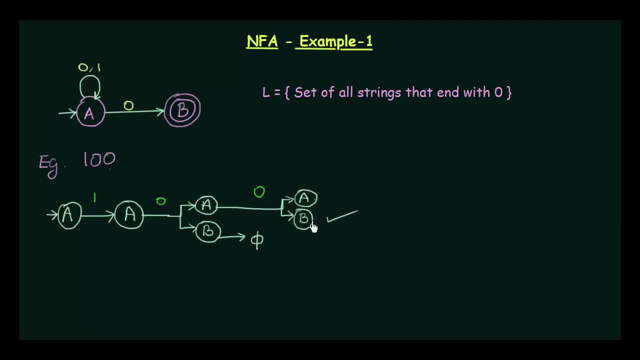 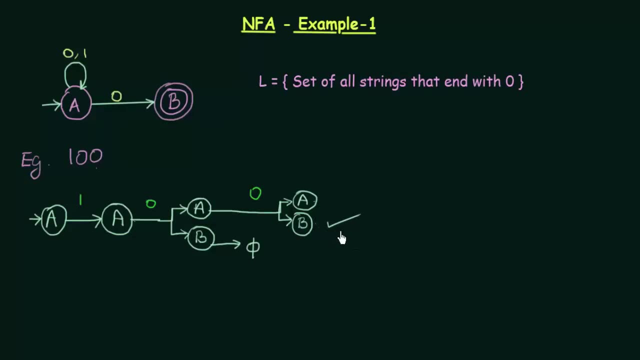 Why? Because if we are in either of the states where one state is an accepting state, then that string will be accepted. Alright, we will write down formally. How can we write down formally? We will write it down after seeing one more example. 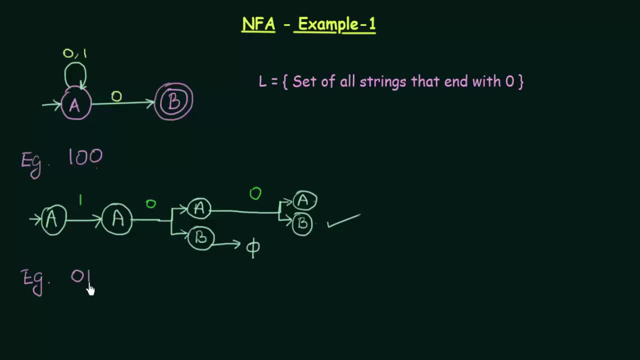 In this example, let me try for the string 0, 1.. Now, should this string be accepted by this NFA? No, Why? This NFA is supposed to accept only the set of strings that ends with 0. But this string ends with 1.. 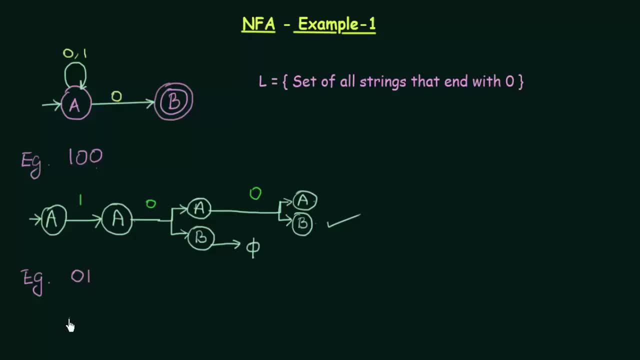 So it should not be accepted. Now let's see how it behaves. We always start from the starting state, that is, state A. Okay, And this is my first input: 0.. Right, My first input is 0.. 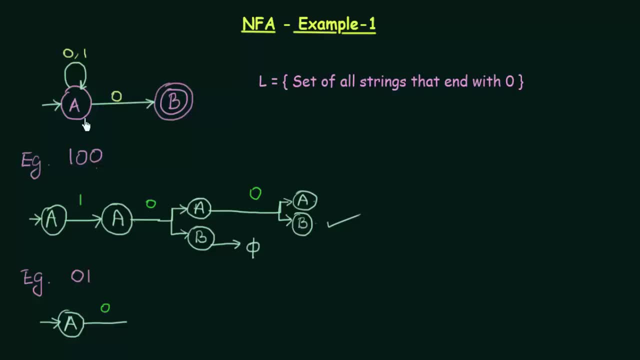 And A on getting 0, where does it go? A goes to A itself and also it goes to B. A goes to A itself and A also goes to B. Right Now I am in two states and I get my next input. 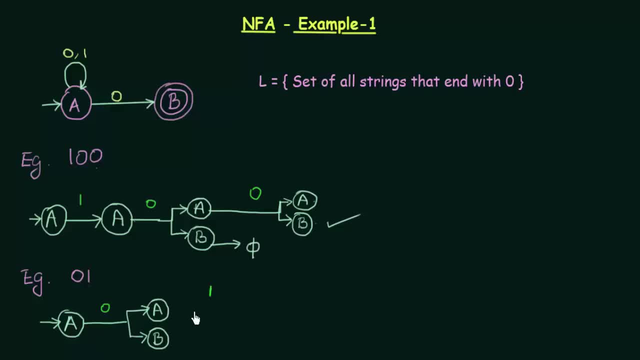 And what is my next input? My next input is: 1. On getting input 1, what happens to these two states? A, where does it go? A- it stays in itself. on getting input 1. A stays in itself. 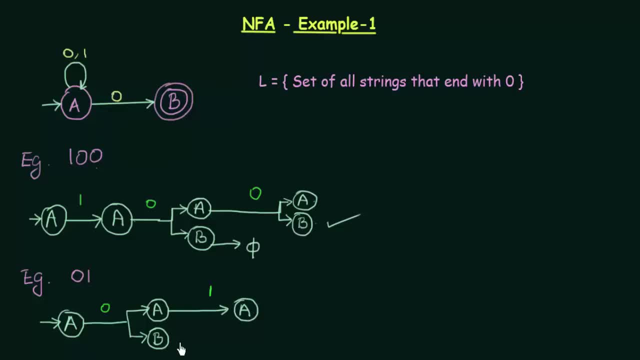 And what about B? On getting input 1, it goes nowhere. So B goes to 5.. Now at the end, I have reached the end of the string. And at the end, what is my position? I am in state A and 5.. 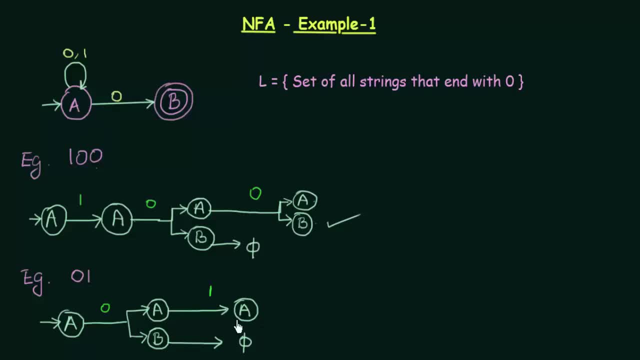 And is state A the accepting state or final state? No, it is not. And 5 is also not the accepting state. So this string will not be accepted. Right, This string will not be accepted. Now how can we formally write down when will a string be accepted? 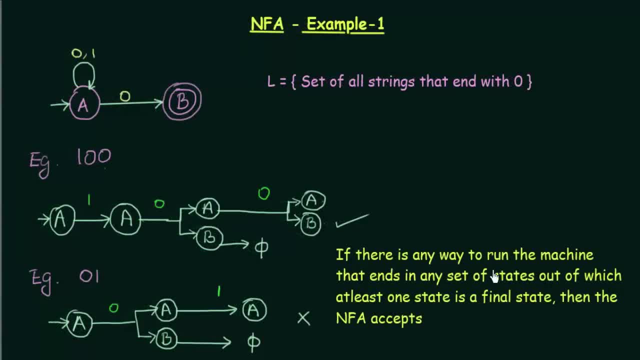 So we can say that if there is any way to run the machine that ends in any set of states out of which at least one state is a final state, then the NFA accepts. When does an NFA accept When it ends in any set of states out of which at least one state is a final state?